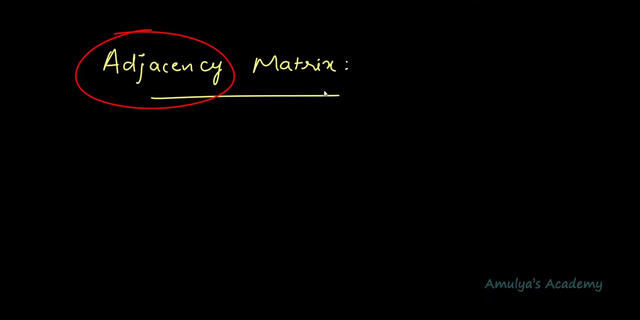 there is an edge between the nodes, or not? Now, what about the matrix? Matrix is a two dimensional array which contains row and column. right, This is a 2 by 2 matrix: 2 row and 2 column. This is a 3 by 2 matrix: 3 rows and 2 column. 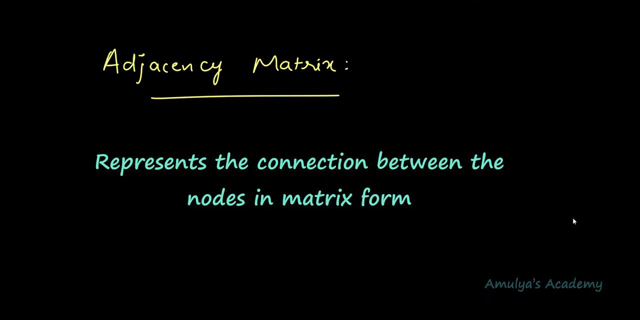 So, in total, an adjacency matrix is a matrix representation of exactly which nodes in a graph contains edges between them. Or in simple words, we can say: it will represent the connection between the nodes in the matrix form. Alright, now we know what is. adjacency matrix is Next. 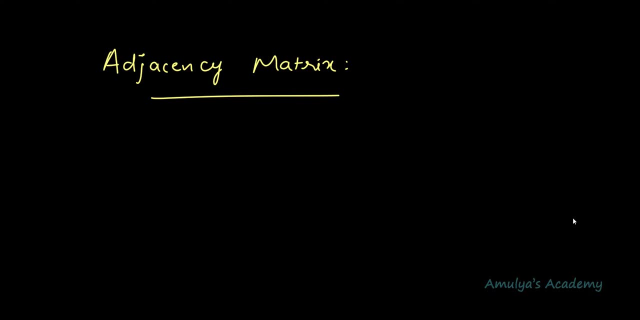 we'll see how to create the matrix In this representation. first we need to create K into K matrix. Here K is the number of nodes present in the graph. First we need to create a K into K matrix and in the matrix both the row and column. 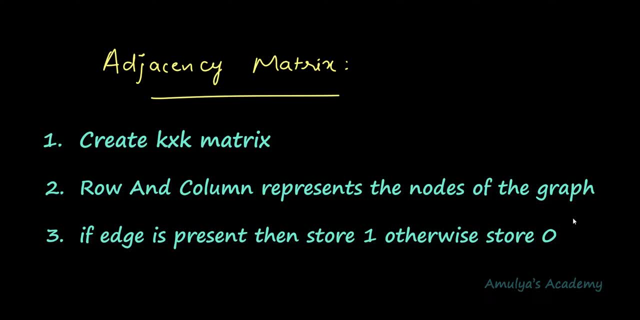 represent the nodes of the graph. If there is an edge between any two nodes, I'll store the value 1.. And if there is no edge between the two nodes, I'll store the value 0.. So matrix will be filled with the 0s and 1s. 0 represents that there is no edge between. 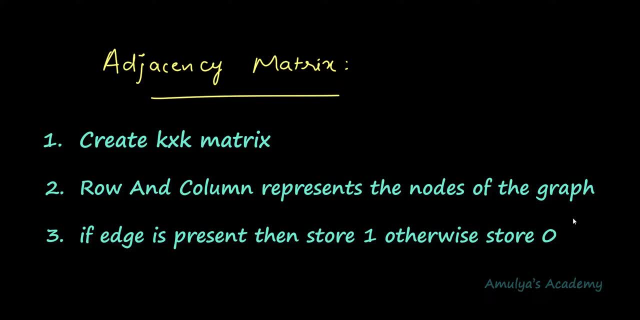 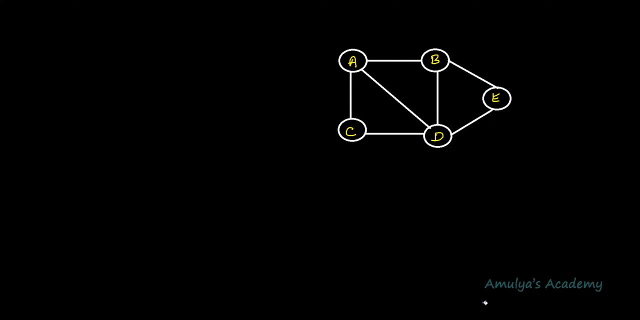 the two nodes. 1 represents that there is an edge between the two nodes. Alright, so. So let's take few example. ok, first, here we have a graph. this is an undirected and unweighted graph. Now, if i want to represent this graph using adjacency matrix, then how to do that? 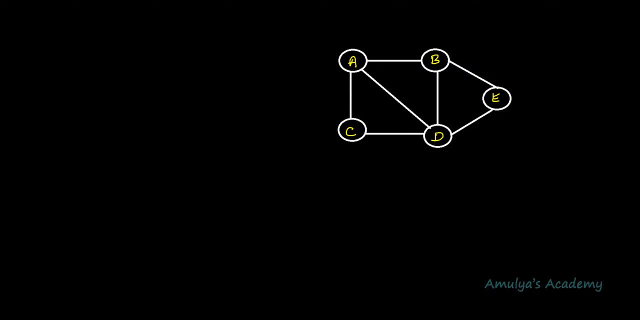 So let's see that the first step in this adjacency matrix representation is: we need to create K into K matrix, and K is nothing but the number of nodes present in this graph. So here, 1,, 2,, 3,, 4 and 5. this graph contains 5 nodes, so first we need to create 5 into 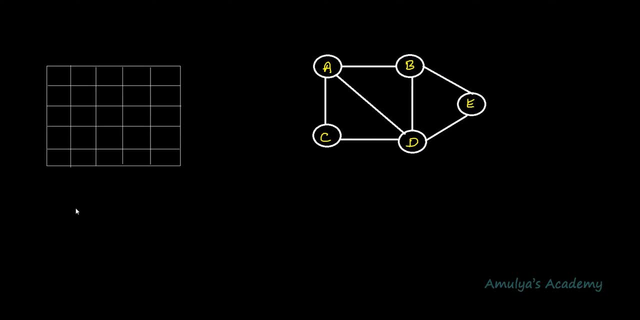 5 matrix. So let's create that. here we have a 5 into 5 matrix. as i said, both row and column of this matrix represent the nodes of the graph. so here i will take first A, B, C, D, E, in. 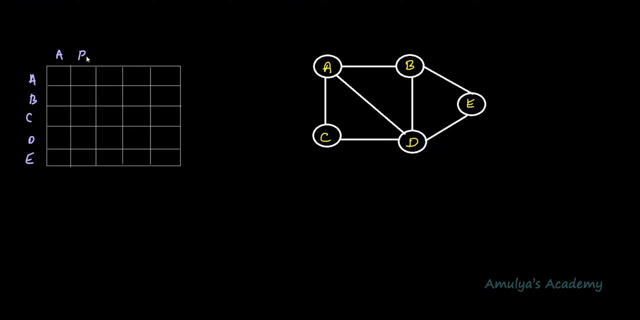 the row the nodes of the graph and here in the column also. i will take A, B, C, D, E. so both row and column will represent the nodes of the graph and in this matrix we need to store 0 or 1.. 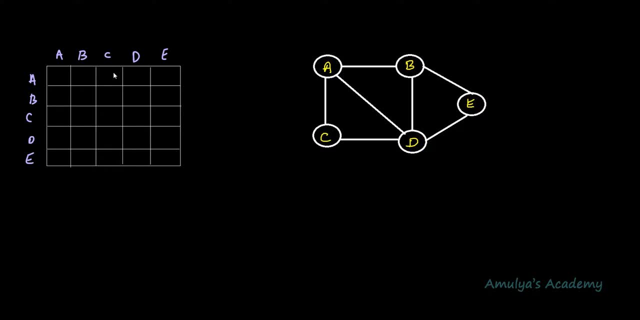 If there is an edge from a node to another node, then i need to represent 1, if there is no edge from a node to another node, then i need to represent 0.. So first let's start from A to A. let's check whether there is an edge from A to A. 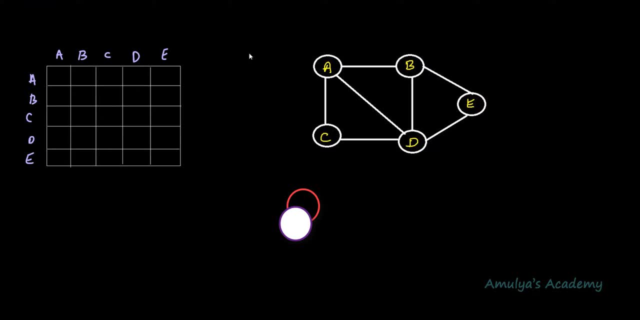 If an edge start from the same node and ends at the same node, then that is called as self loop or self edge. Here we don't have that right. we don't have any edge from A to A, so that's why here i will store 0.. 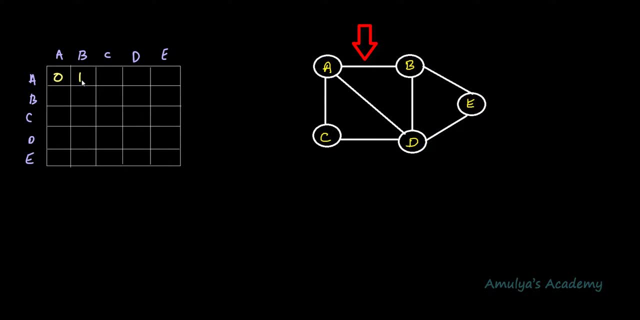 Next A to B. here we can see there is an edge. so i will store 1,. A to C. yes, there is an edge A to D. yes, there is an edge A to E. no, there is no edge from A to E, right, that's. 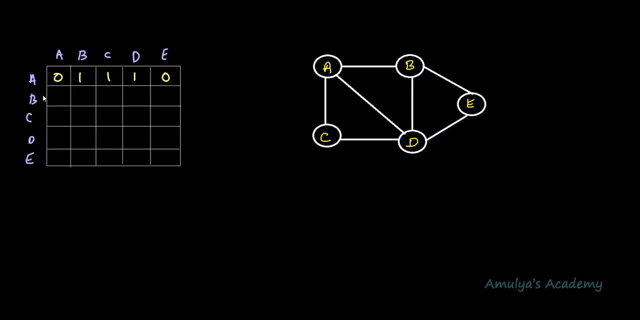 why 0.. Next let's move on to the next row: B to A. yes, here we can see this is an undirected graph. So we have an edge from B to A only. So here 1, B to B. no, we don't have any self edge here. B to C: no. B to D: yes. B to E: yes. 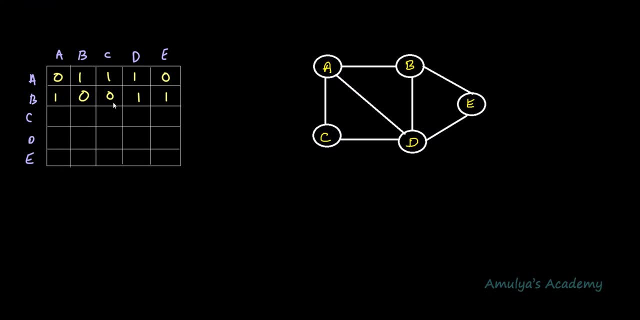 that's why store 1.. Next move on to the next row: C to A. yes, there is an edge. C to B. no. C to C. no C to D. yes. C to E. no. Next D: D to A. yes. D to B. yes. D to B. no D to A. yes. D to B. yes. D to B. yes, D to B. 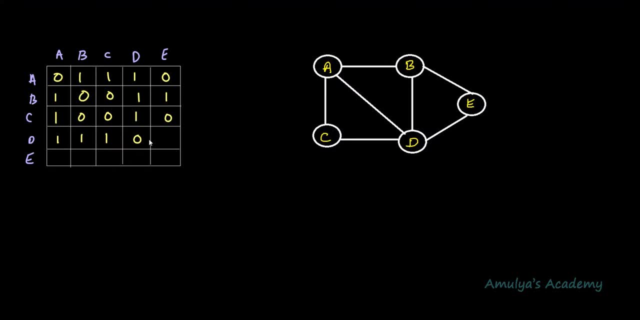 yes D to C. yes D to D. no D to E. yes Next E to A. no E to B. yes E to C. no E to D. yes E to E- no. So this is the adjacency matrix for this graph. 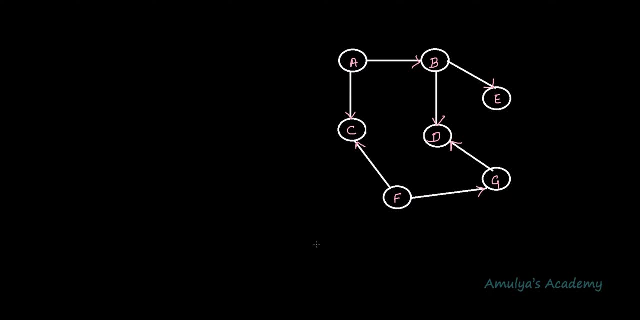 So next let's take another example. let's take a directed graph Now. first step in this representation is We need to create K into K matrix, where K is the number of nodes present in the graph. So here 1, 2,, 3,, 4,, 5,, 6, 7.. 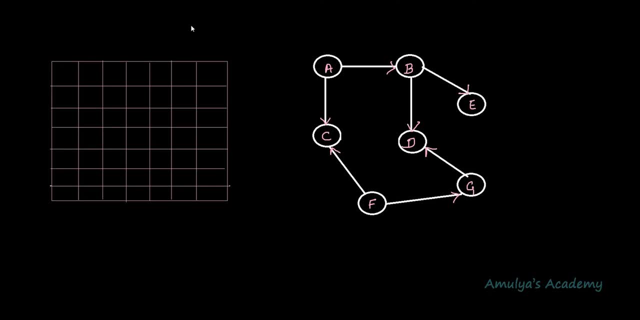 So first we need to create 7 by 7 matrix. So here we have 7 by 7 matrix, so you can take this in any order, ok? So let's check whether there is an edge from A to A. no, A to B. yes, A to C. yes, A to D. 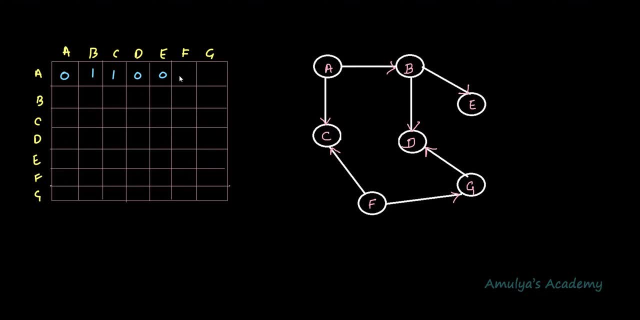 no A to E, no. So let's check whether there is an edge from A to A. no A to B, yes A to C, yes A to D. no A to E, no A to F, no A to G, no. 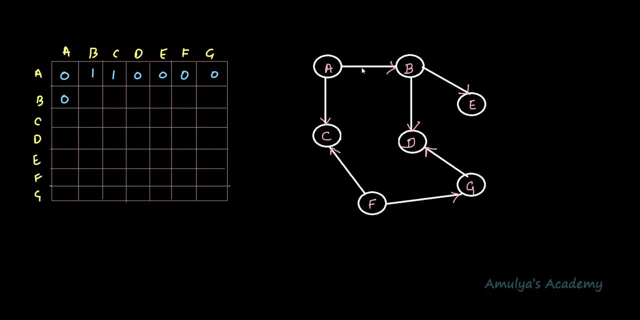 Next, from B to A. no, because this is the directed graph. here you can see there is an edge from A to B, but there is no edge from B to A. B to B: no. B to C, no. B to D. yes. B to E: yes. 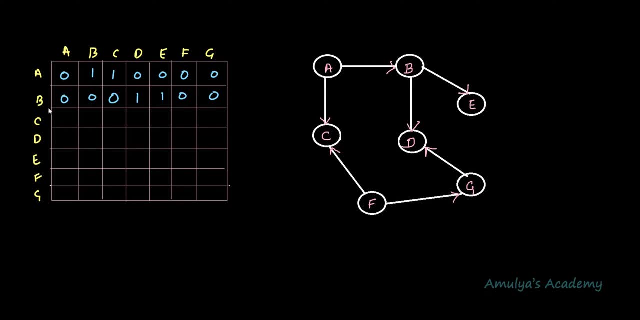 B to F. no B to G no. Next from C: C to A. no C to A. no C to B. no C to C. no C to D. no C to E. no C to F. no C to G no. 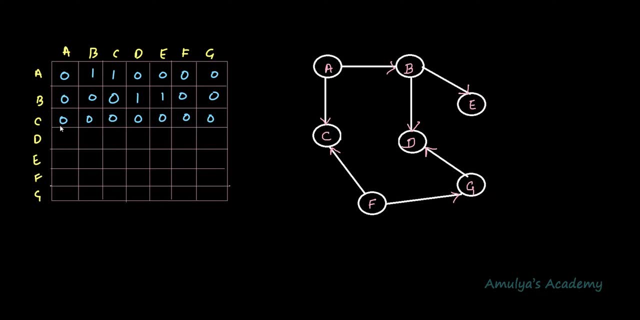 Next from D So D to A. no D to B. no D to C. no D to D. no D to E. no D to F. no D to G. no Next E From E to A. no E to B no. 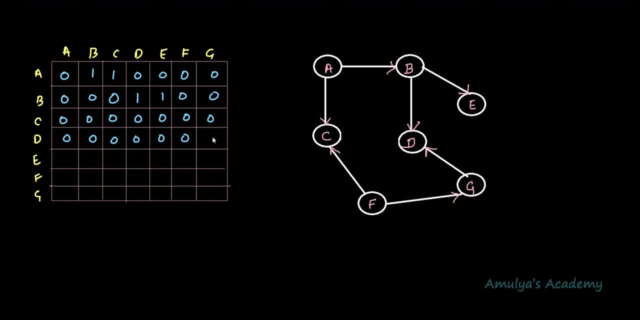 E to C, no E to D. no E to E, no E to F, no E to G. no Cool Next E From E to A. no E to B, no E to C, no E to D no. 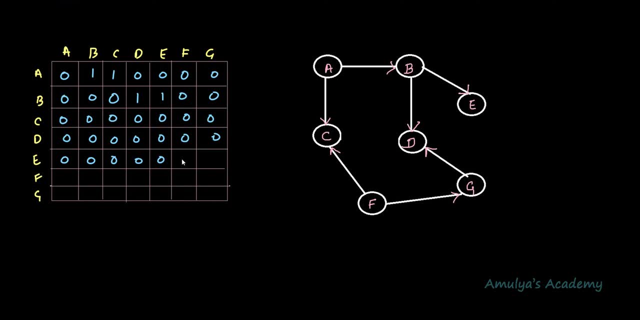 E to E. no E to F. no E to G. no E to G. no E to F. no E to G. no Next F: F to A. no F to B. no F to C. yes F to D no. 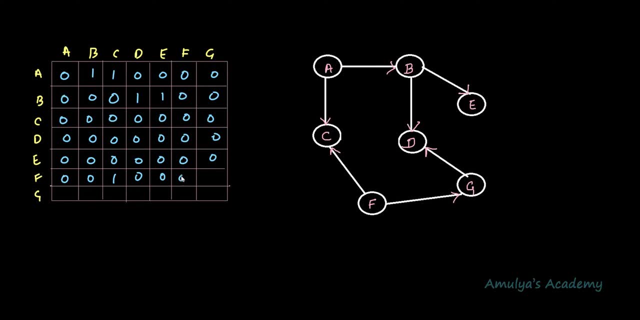 F to E: no F to F, no F to G. yes, There is an edge. right Next from G: G to A, no G to B, no G to C, no G to D. yes, Here there is an edge. 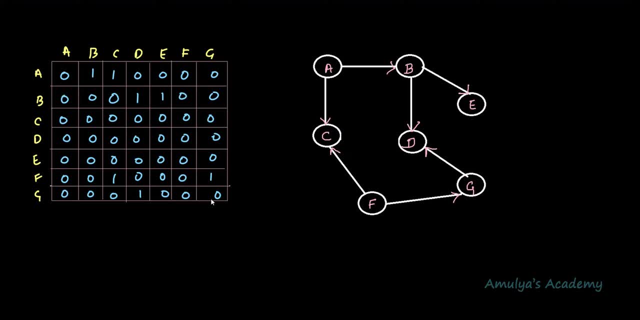 G to E. no G to G. no G to F. no G to G. no, This is the adjacency matrix. If there is an edge, you need to represent it as 1.. If there is no edge, you need to represent the value 0.. 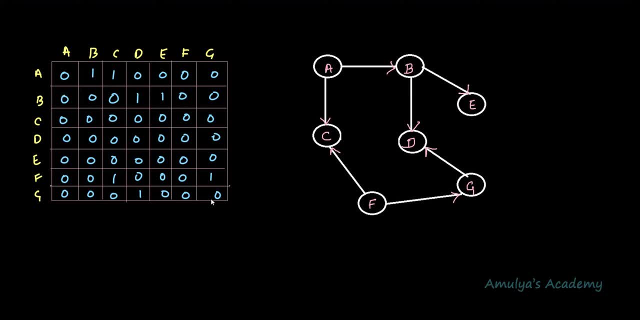 And in the row and column you need to take the nodes of the graph. Alright, So this is about the directed graph and undirected graph, But what about the weighted graph? In the weighted graph, every edge will be associated with an value, right? 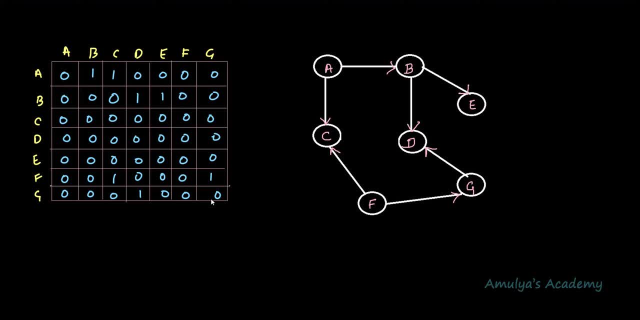 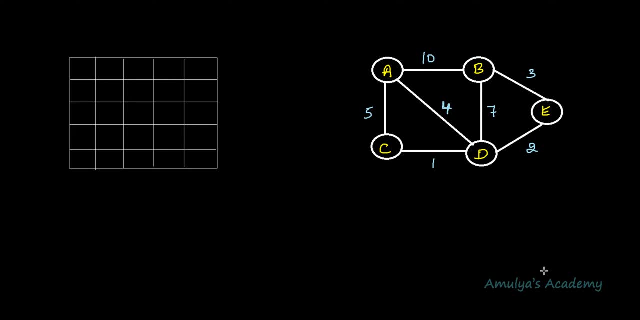 Then how to represent that in the adjacency matrix form. So let's take another example. Here we have a weighted graph. Let's see how to represent weighted graph using adjacency matrix In unweighted graph. what we did is: if there is an edge from a node to another node will. 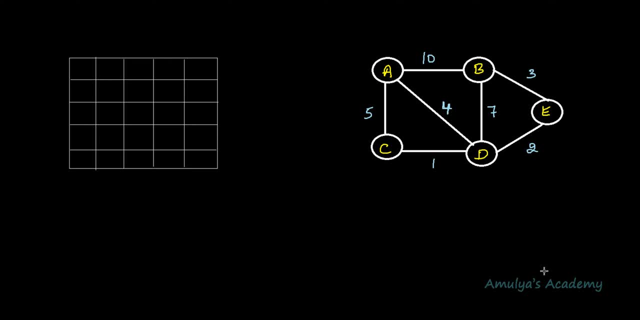 represent or will store the value 1.. In the weighted graph, what you need to do is, if there is an edge from one node to another node, instead of storing 1, you need to store the weight of that edge, Cost of that edge And rest everything as 1.. 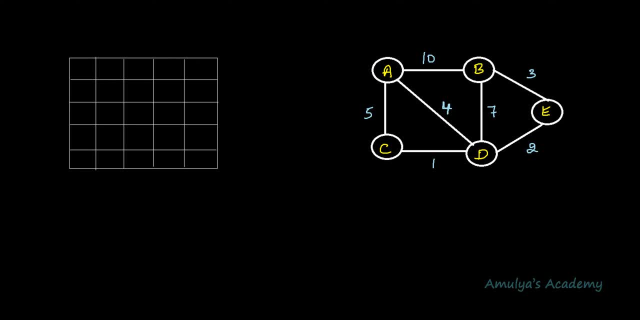 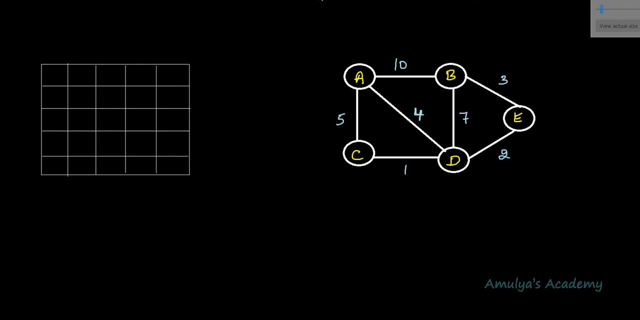 And rest. everything is same. You need to create K into K matrix. K is nothing but the number of nodes present in the graph. So here this graph contains 5 nodes, so we created 5 into 5 matrix. Then here write down the nodes: 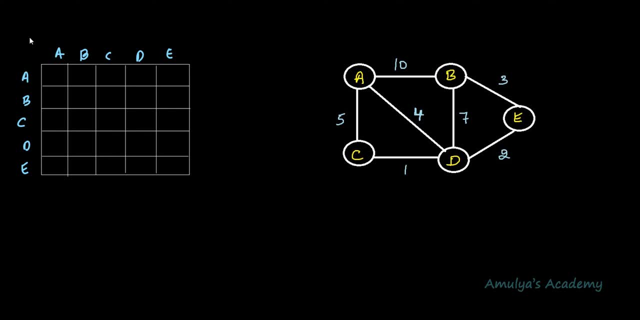 Then let's check whether there is an edge from A to A. No, So 0.. Let's check from A to B. Yes, there is an edge from A to B. Now, instead of storing 1, we need to store the cost of that edge. 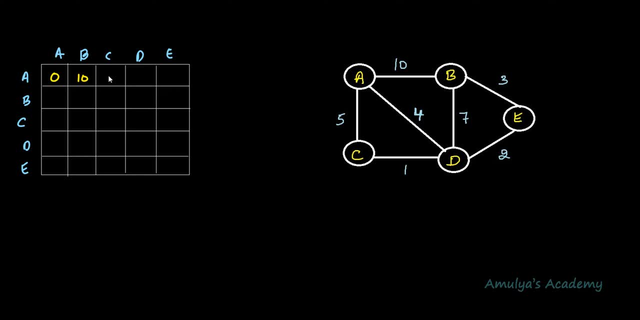 That is 10.. Next, A to C: Yes, so 5.. Store the cost. A to D: there is an edge and cost is 4.. A to E: there is no edge, so store 0.. Now B to A: 10, B to B: 0, B to C: 0, B to D: the cost is 7, B to E: 3.. 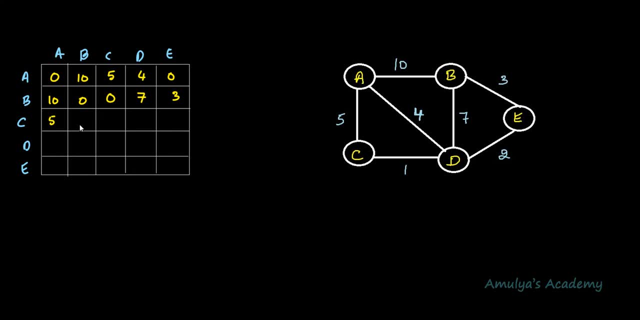 Next: C: C to A: cost is 5,. C to B: there is no edge. C to C: no. B to D: there is no edge. B to C: 0.. C to D: cost is 1,. C to E: there is no edge. 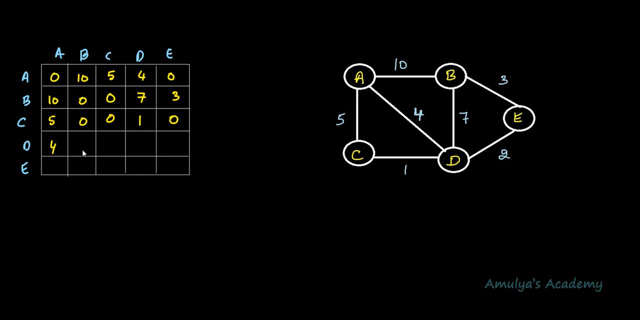 D to A cost is 4,. D to B cost is 7,. D to C cost is 1, D to D: 0,. D to E cost is 2.. Next, E to A: 0. there is no edge. E to B cost is 3.. 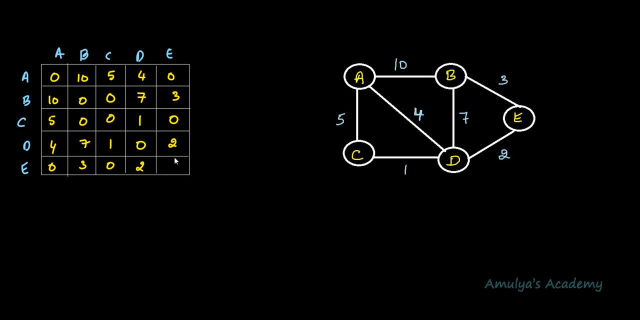 no edge. E to D cost is 2, E to E: 0.. This is the adjacency matrix In the weighted graph. when there is an edge from a node to another node, instead of storing one we need to store the weight or cost of that edge. I hope now you understood how to create the adjacency. 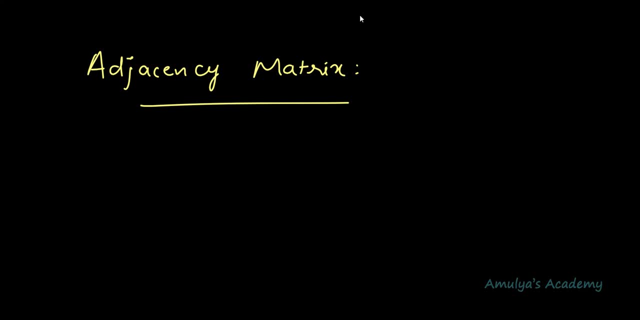 matrix for given graph and one of the interesting thing about this adjacency matrix representation is just by looking at the adjacency matrix you can say whether the graph is directed or undirected. Also, in some time you can say whether that the graph is weighted or unweighted. 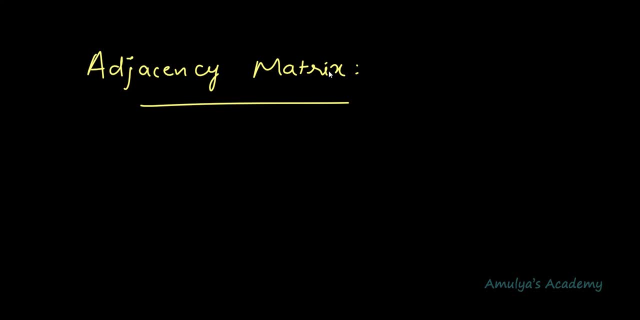 also, If the values on the both these sides of main diagonal of an adjacency matrix are same, then that matrix is symmetric and that symmetric matrix represent the undirected graph, For example. here you can see this matrix. here, in this adjacency matrix, the values on both the sides of the main diagonal is same. 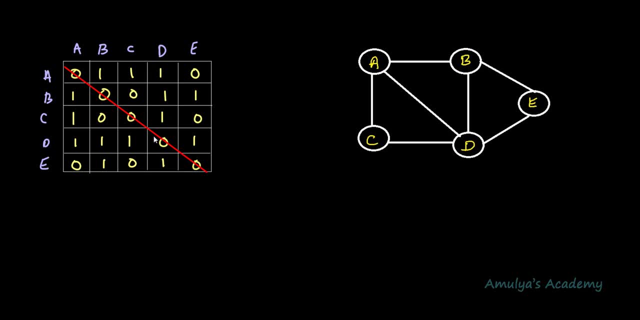 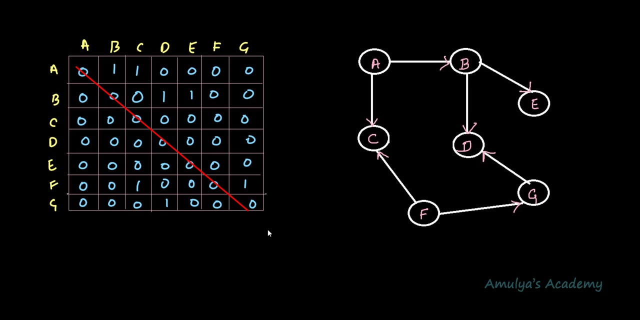 here you can see, right, it is symmetric. by looking at this matrix, i can say this matrix is representing an undirected graph. in the directed graph here we have. here you can see it is not symmetric. that's why i can say this is representing the directed graph. 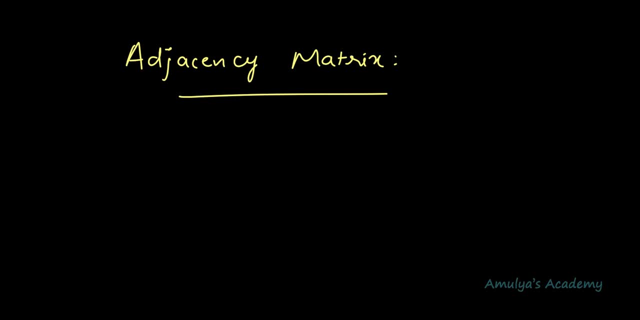 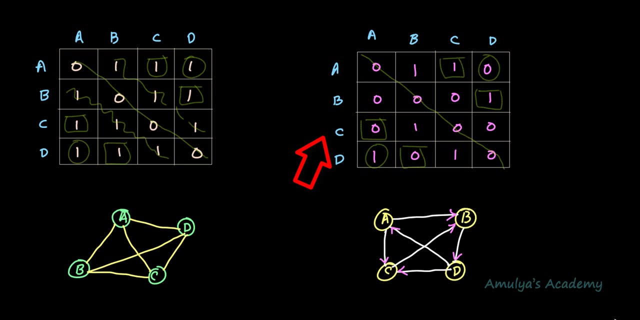 So when adjacency matrix is given, you can say whether that matrix is representing the directed graph or undirected graph. here this is representing directed graph and this is representing an undirected graph. in the undirected graph, values of the both the side of the main diagonal is symmetric, is same, and by looking at the adjacency matrix you can also say whether 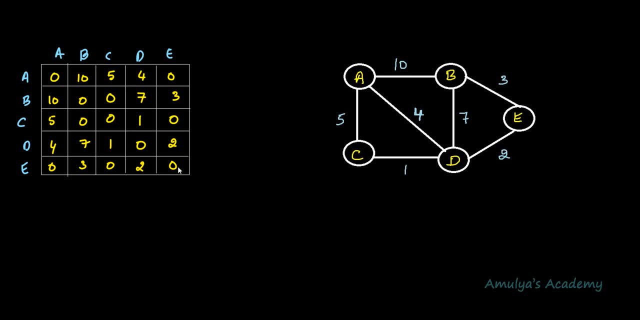 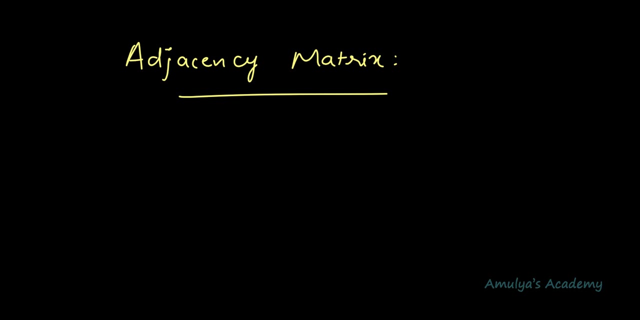 that graph is weighted or not, because in the weighted graph will represent cost of edge right. but if the cost of all the edges of graph is one, at that time i can't say whether that adjacency matrix is represented or not, but usually will have different cost for different edge right in the weighted graph. so usually 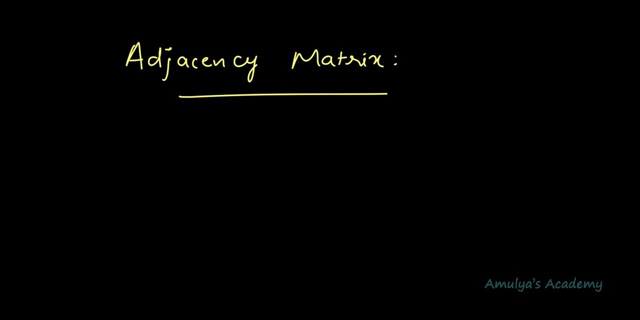 you can say whether an adjacency matrix is representing the weighted graph or not. here you can see it is representing the weighted graph, all right, so this is about the adjacency matrix. here i want to implement graph using python programming language. right? i want to create adjacency matrix to store graph in python. 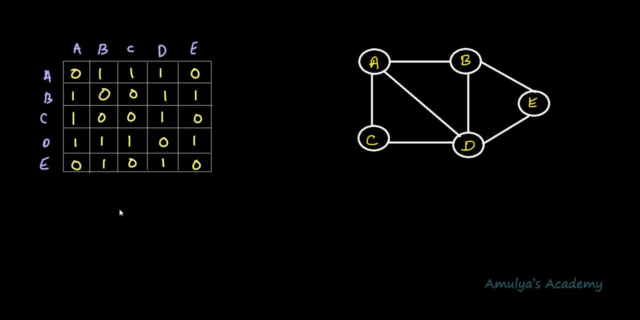 then i can use nested list for that. here to create the matrix, i can use nested list and also we can create a separate list to store the vertices or the nodes of the graph, like this: a, b, c, d, e. a list index will be start from zero, two, three, four. then to store this: 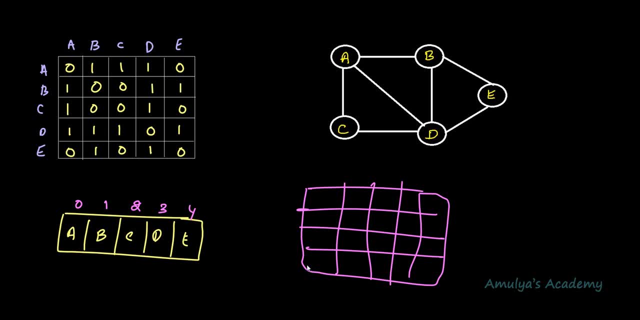 matrix i can create a nested list like this and here also index will start from zero, two, three, four. so in python for the adjacency matrix we can represent like this: for matrix we can use nested list and we can take another list also to store the vertices or nodes of. 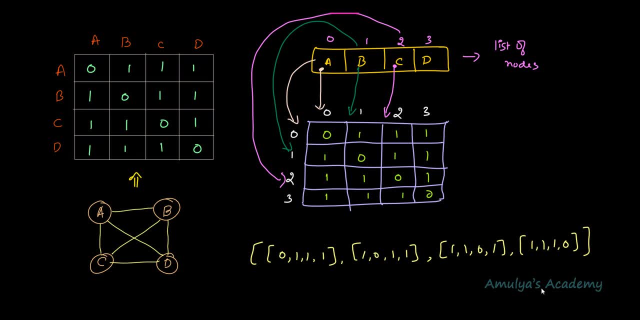 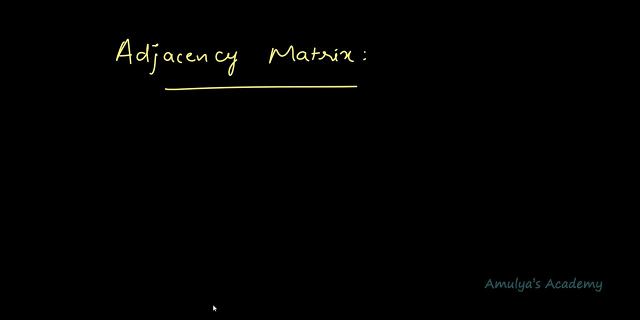 the graph like this: here you can see the representation. all right, so this is about the adjacency matrix, and in the next tutorial we'll talk about the adjacency list, why we have different graph representation. why can't we just use adjacency matrix to store the graph? why we need to study adjacency list also? that is because every method has its own advantage. 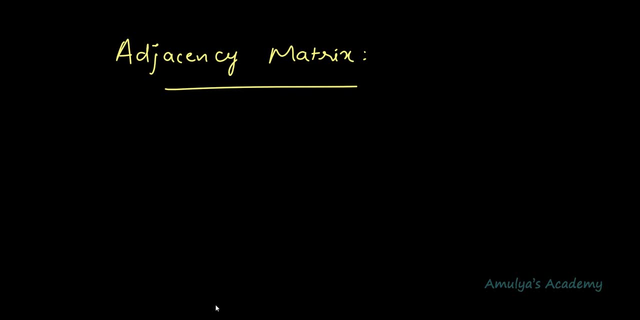 and disadvantage here. adjacency matrix is easy to follow and represent. the adjacency matrix is representing the connection between the nodes, whether there is an connection between the node or not. the question is this: whether there is an edge between the nodes or not, the answer for this question is yes or no. but in the adjacency matrix, what we are doing, 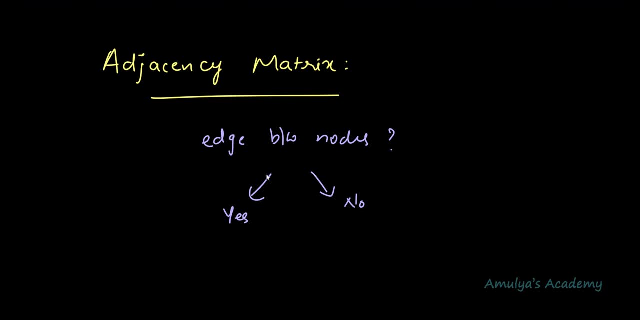 is, we are storing the result for both the nodes and we are storing the result for both the nodes. in this condition, if there is an edge between the node, we are storing the value one. there is no edge between the value, we are storing value zero at that time. so we 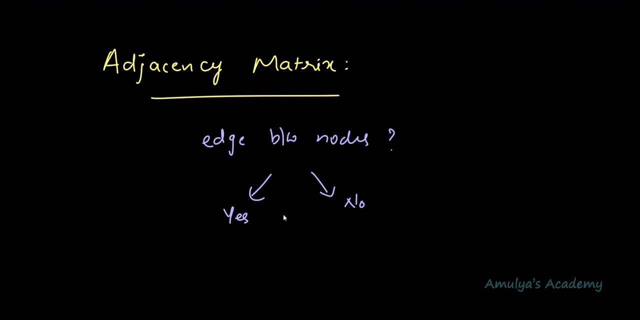 are representing or storing the result for both the cases. if there is an edge, we are storing some value. if there is no edge, then also we are storing the some values. that's why we are using more memory space. if we are using the dense graph, then it is okay because 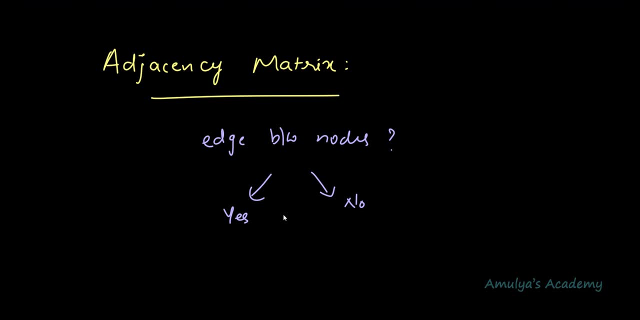 we don't have too many zeros in the adjacency matrix- okay. that's why it is okay. but in this sparse graph we will have too many zeros and we are storing that zeros in the memory. that's why we are wasting the memory. a graph in which